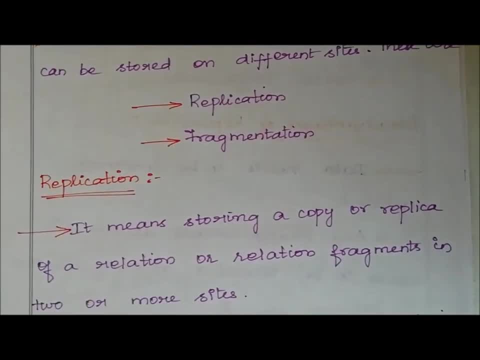 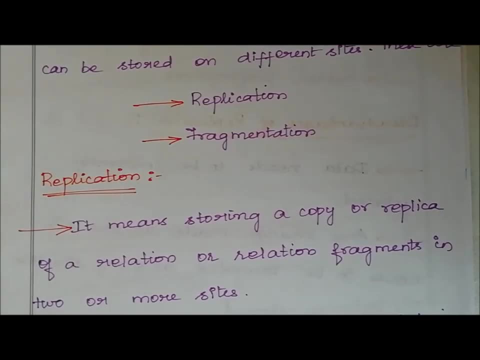 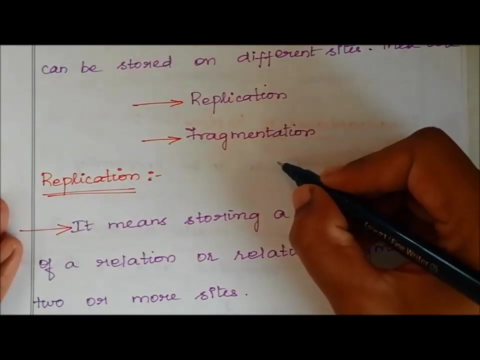 What is replication? Okay, so replication it means storing a copy or replica of relation or relation fragments into our most sites. Okay, so the copies of records are stored in different sites? Okay, in a particular database, for example, I am going to store 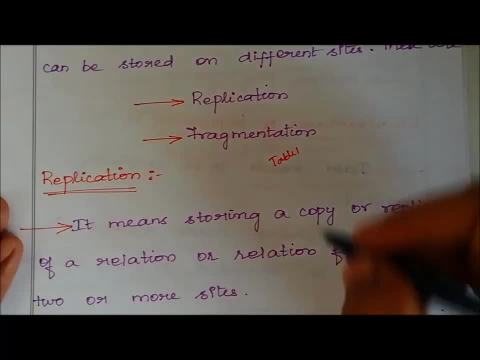 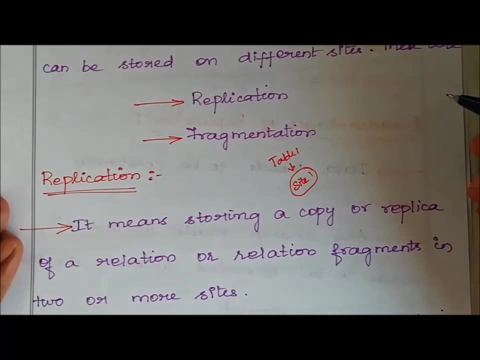 table 1.. What am I going to do with table 1? I am going to store it. To store it, I am going to store table 1 in site 1.. As well as suppose table 1 is stored in site 1, I. 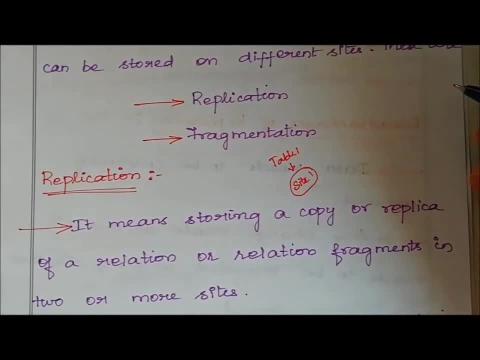 am going to store it in site 2,. so what is the? network failure or system failure? If there is any network failure or system failure, I can't do anything. I can't retrieve that table. What I am going to do for that is, I am going to store two or three sites. 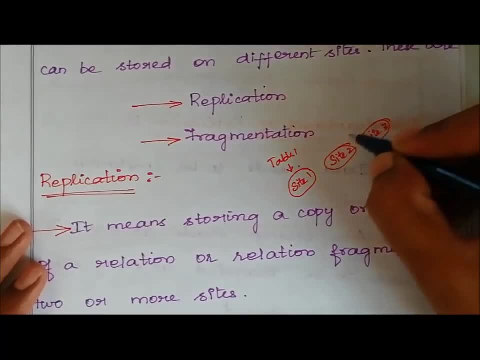 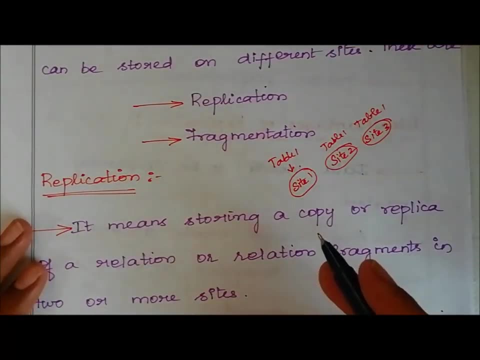 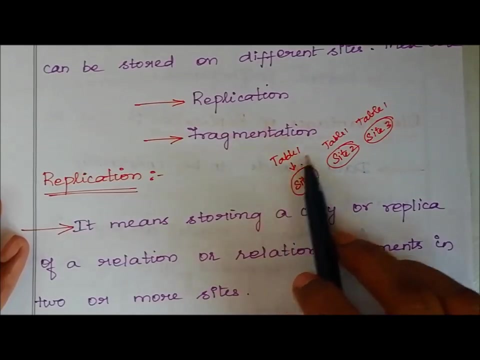 in maining and a copy of the same site and store it So I can retrieve that particular record, particular table- table 1, if there is any system failure or network failure. When there is a network failure or system failure, I am able to retrieve that table. 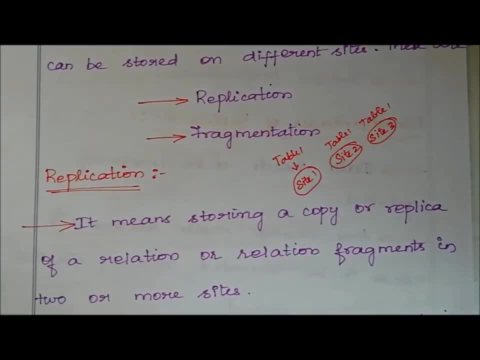 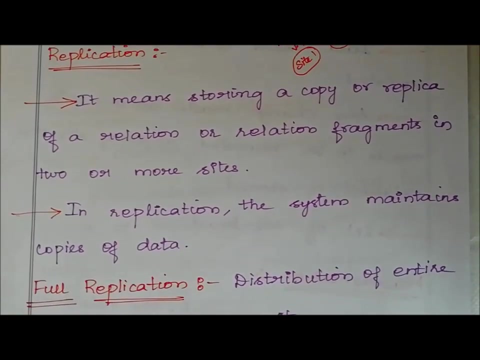 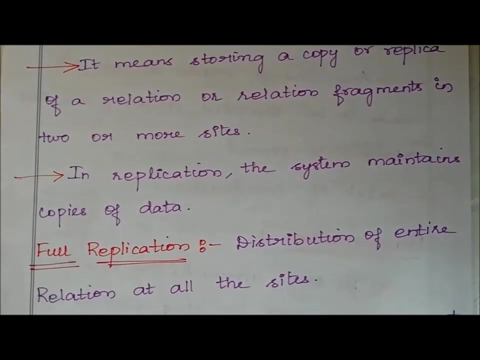 that is table 1.. Okay, so that is storing of storing of records, a copies of relation. okay, in different sites, sorry, the in different sites, that is, in different pieces. okay, that is replication. in replication, the system maintain copies of data. okay, so, different copies of data system, nothing but pc, or we can say site. okay, so there are two types. 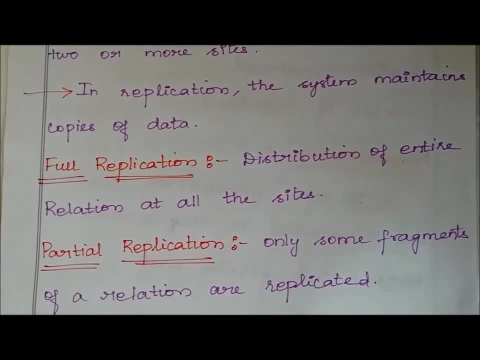 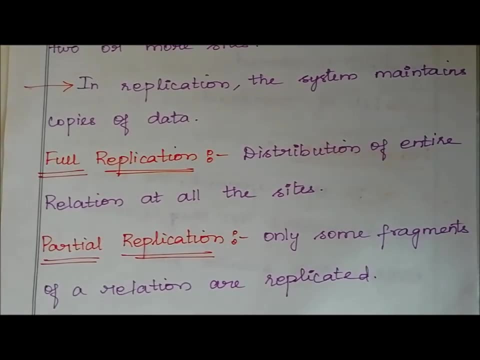 in replication. first one is full replication and second one is partial replication. full replication is distribution of entire relation, at all the slides or at all the sites. okay, so entire table. you know my one do a lot of sites in store, for no, I'm Dana. okay, entire table. copies of: 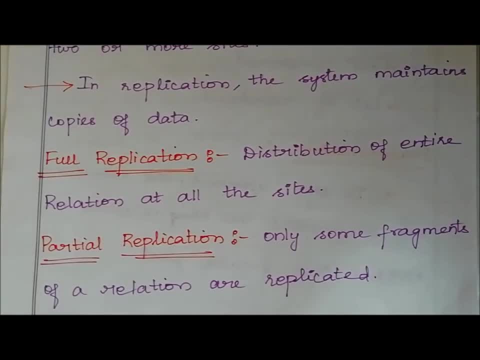 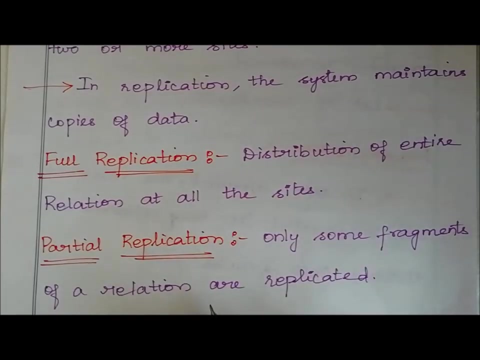 the entire table. it's stored in different sites. not a minus, or that is full replication, partial application, only some fragments of the relation or replicator: okay. so if we store only some of the fragments of that relation okay in the in different sites, then it then it is called partial replication, okay, full. 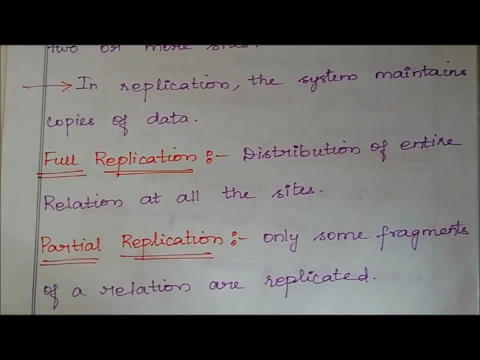 replication and in a particular entire relation, you know when the last it's in store for no, I'm Dana. that is full replication, partial replication, not so the fragments. much to the menopause row store panorama, different sites is to a panorama, Dana. okay, for example, table one of these example. 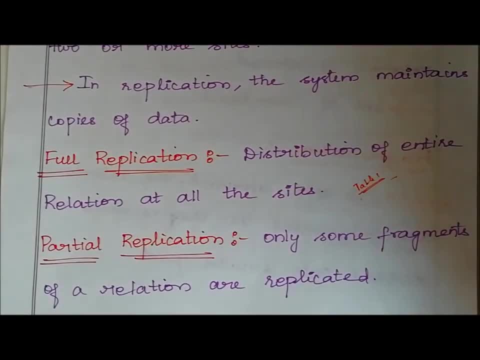 I think not table one number, the complete and I end up under a line of the three fragments are. can watch my fragment one, fragment two, fragment three. okay, so smaller parts of a table, the fragments so far in this villa in the in the fragments element, the right records. allow me now on this side, one up to site, the end working. I. 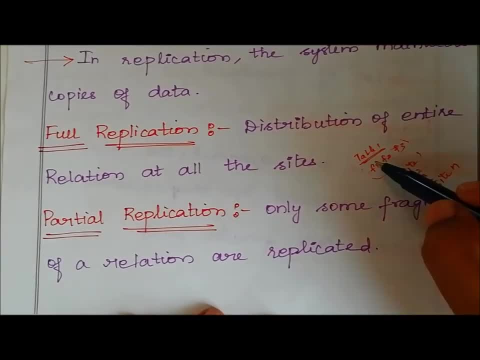 like the Lena's, to a panorama that is full replication, partial replication, not in the important, a fragment to the way, no matter is a loss and I, like the personal, personal, I'll be now the fragment to a mutton and I found a loss. it's neither to site one to 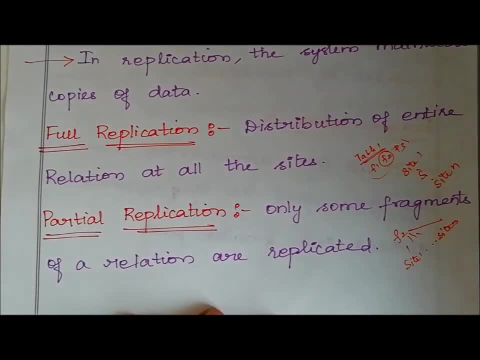 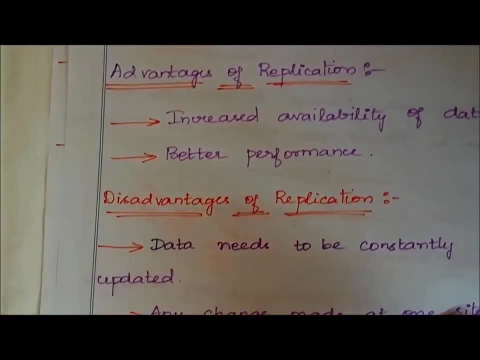 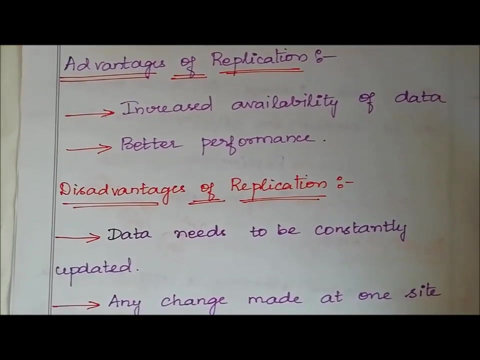 say the endless to a panorama, okay. side one to over you in a school pendant. that is called as partial replication, okay. so let's see that. bandages of replication- okay. increase availability of data. so laws are not only in our therapy: data cutting- okay, that is in this. availability of data, better performance, okay. 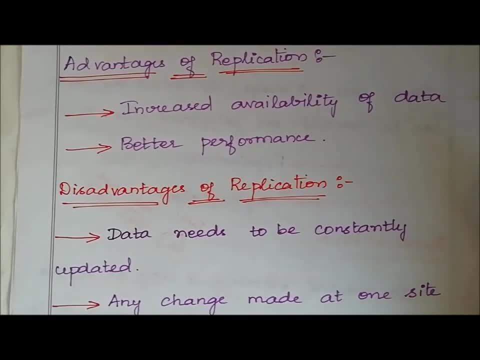 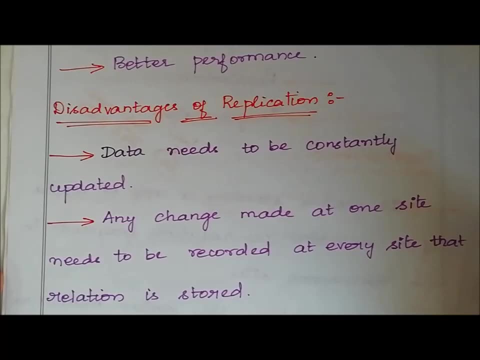 so normally my multiple copy store pandan Allen will give a better for performance can carry okay. and then advantages of application. sorry, this advantages of application. data needs to be constantly updated. for example, in multiple copies is no more store panikin Allah site. one lay down. 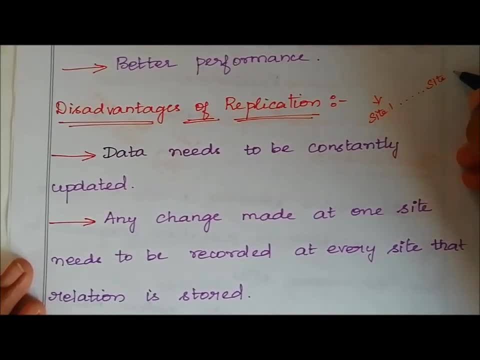 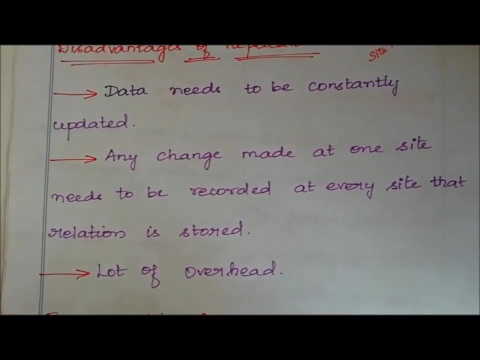 okay, that change should be updated in all the sites. okay, so in all the sites the changes should be updated. okay, so this is a disadvantage. any change made at one site need to be recorded at every site that relation is stored, so where all the particular relation is stored. 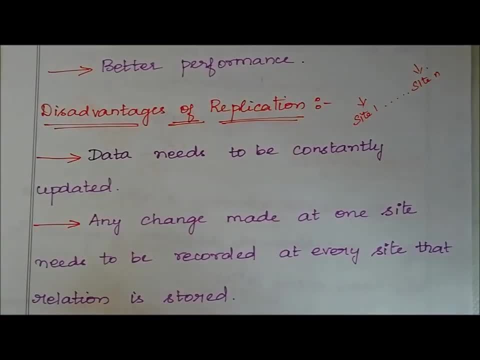 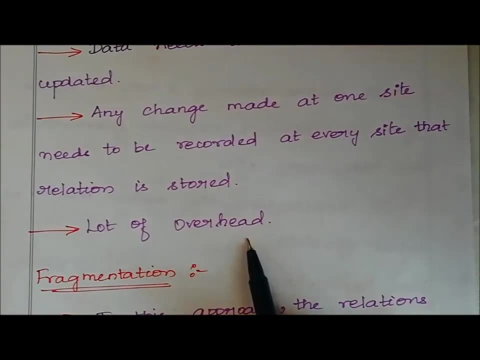 in which site all the particular relation is stored in that site. in which site all the particular relation is stored in that site. okay, so lot of overhead, definitely what we have to do. this is a big job without changing in one site what we have to do in all the sites. 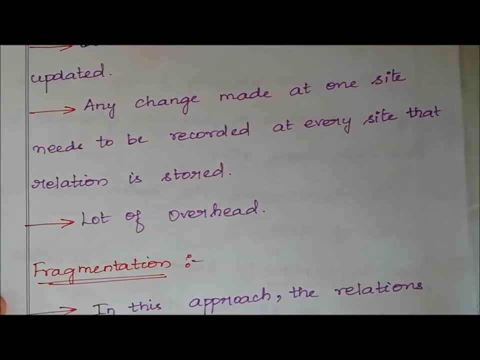 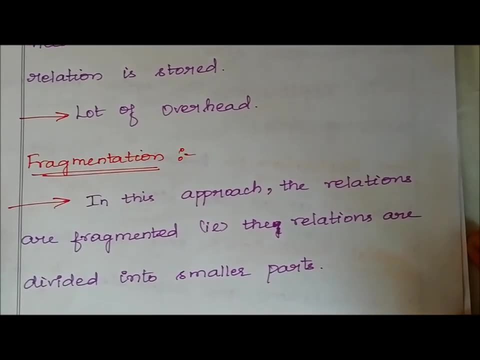 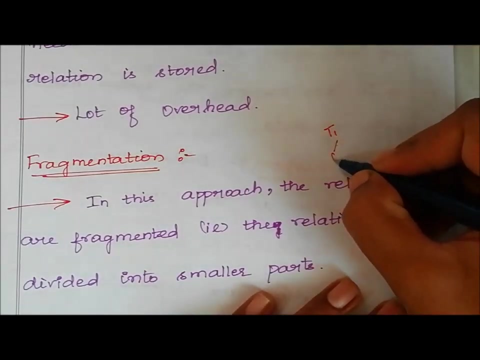 change, so lot of overhead in replication. okay, let's see the second type in distributed data storage, that is, fragmentation. in this approach the relations are fragmented, that is, the relations are divided into small, smaller parts. that is, we can take a table T1 so we can take fragment 1. 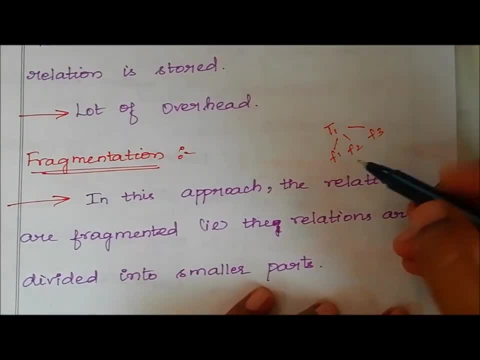 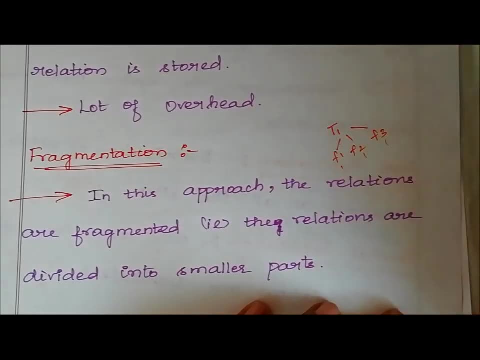 fragment 2. fragment 3. fragment 4. fragment 5. fragment 6. fragment 7. fragment 8. fragment 9. fragment 10. okay, so we're reading over season. I still ponding, so that is your phone. were a site left to our site, life three was like the same- less when the man is. 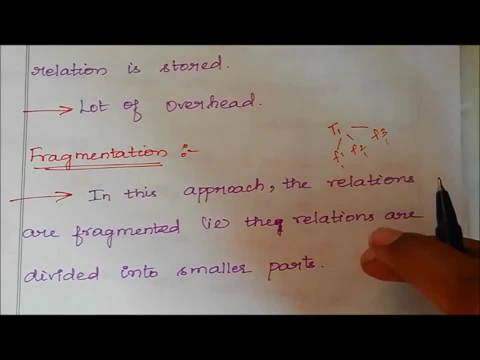 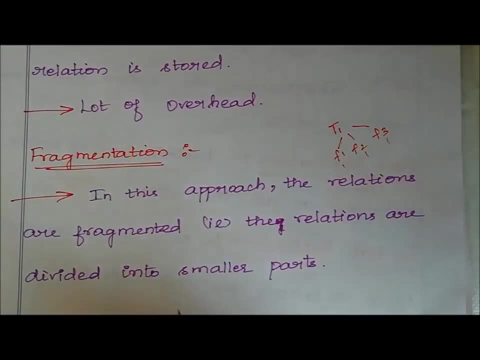 open and that process is called fragmentation. fragmentation of a relation of another. now, in this, smaller parts are divided, punish upon other. that is the F1, F2, F3- a Monday, wait for your children- fragmentation, okay. in this approach, the relations are fragmented. that is the relation, that is. 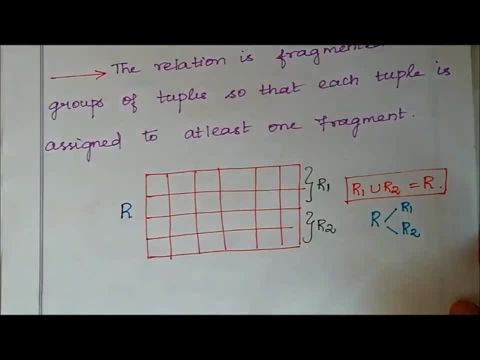 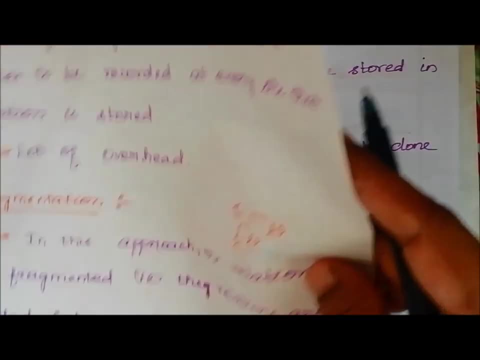 divided into smaller parts, okay, and then we also just have a different point of fragmentation of each of the fragments are stored in different sites. okay, I must money, with no device, and the fragments and I'm on the table, wanna your phone. you have to have three and 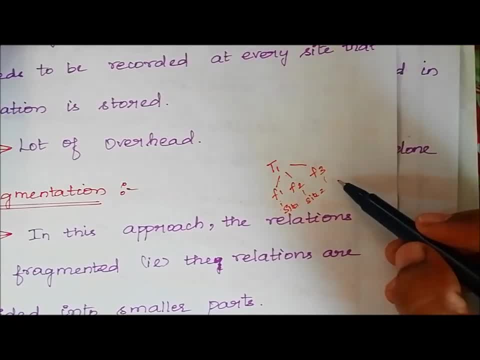 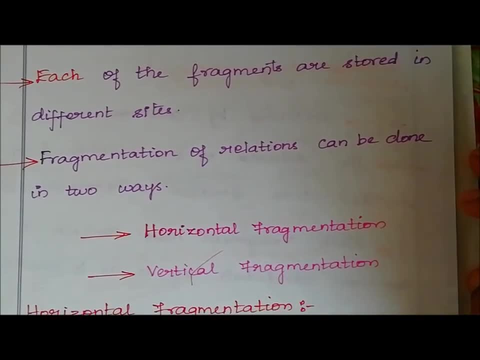 I'm a device, for it was fact much over the site, one less to upon run off our fragment to and an up under site tool or sport contract, fragment 3 and an up, and I say threadless to upon ok. so the each of the fragments are stored in different. 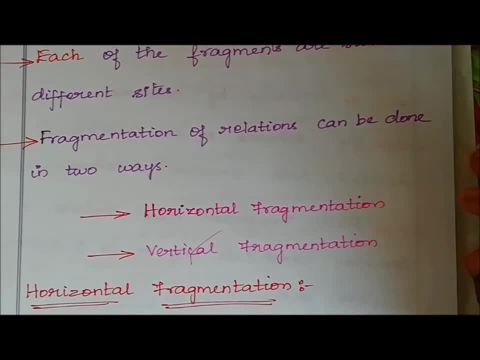 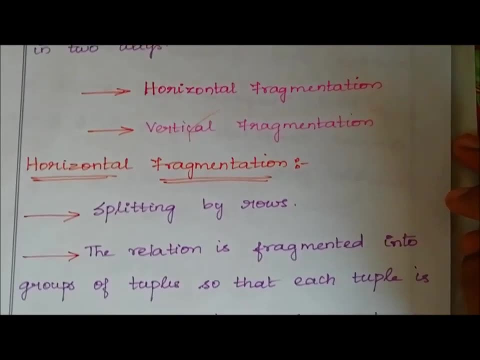 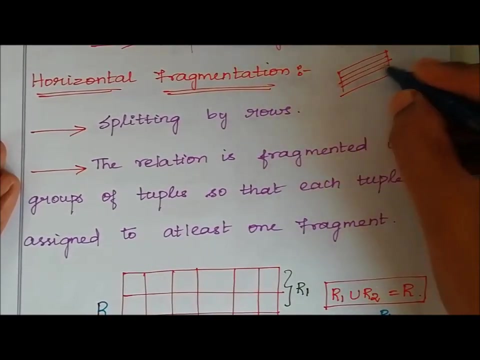 sites. ok. third point is fragmentation of relations can be done, and two ways: ok, fragmentation, and second one is vertical fragmentation. Let's see what is horizontal fragmentation, For example. this is the horizontal fragmentation. So like this, for example, I will divide the first 4 rows. 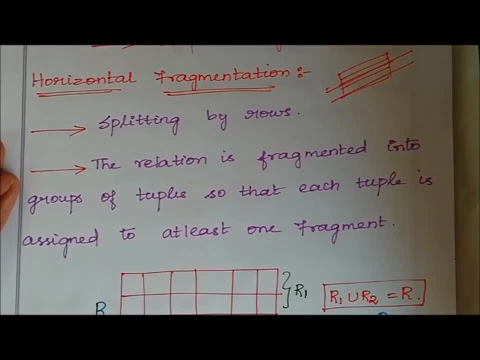 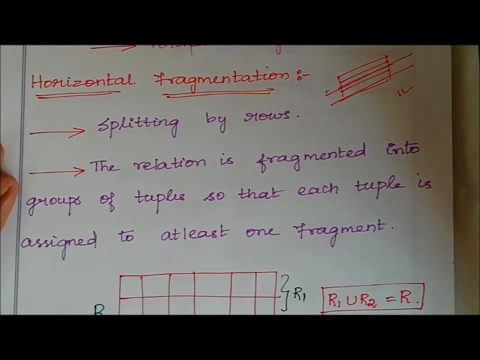 into a fragment, I will divide the next 4 rows into the next fragment. For a small table, if it is in lakhs, if there is 1 lakh of rows in a table, then I will divide into 1000.. For 10k: I will divide the first 10k into a fragment. 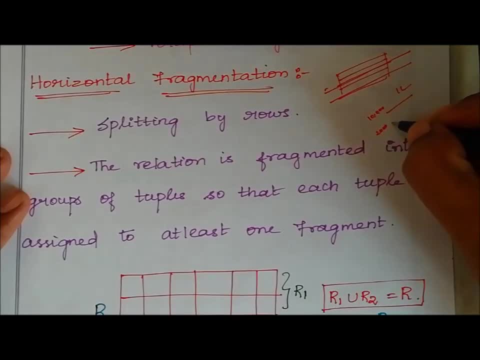 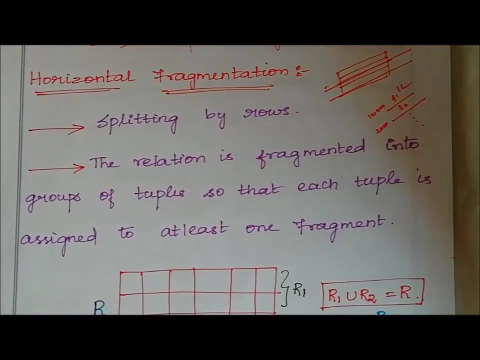 Next is 20,000.. That is, from 10k to 20000. I will divide the next fragment into 4 Lakhs. for another 1 lakh size, 10 fractions will be equal to a Lakh. So like this we are dividing it into another fragments for horizontal fragmentation. 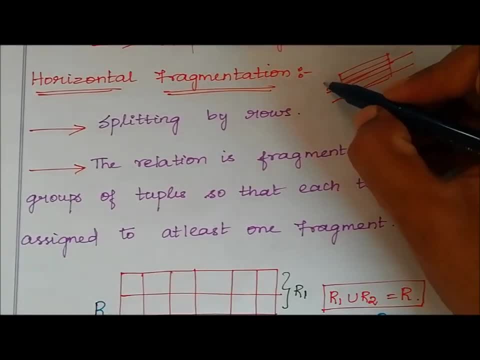 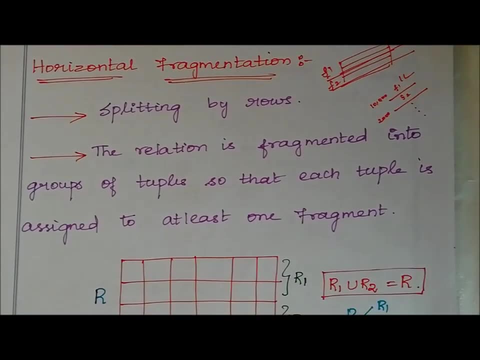 If the table has 8 rows, then, whether it be the next 4 rows or the next 4 rows´ being a fragmentation, I will divide them into horizontal fragmentation, where it is splitting by rows. okay, The relation is fragmented into groups of 8 rows. 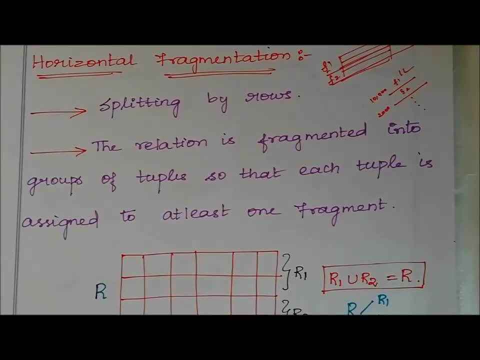 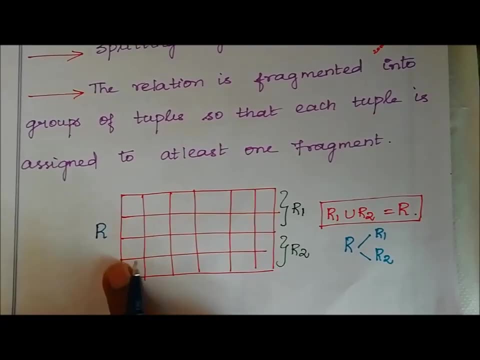 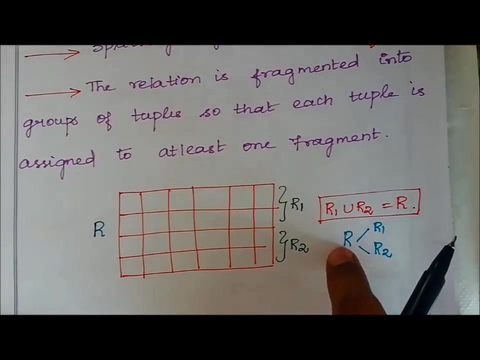 so that the each table is assigned to one, assigned to at least one fragment. okay, well, for example, you do a table relation or relational table. okay, so relation are in a pendant, or one or two, not divide. panda, I did lending, combine panna. again, I should get the same. relation are okay, so are one. or 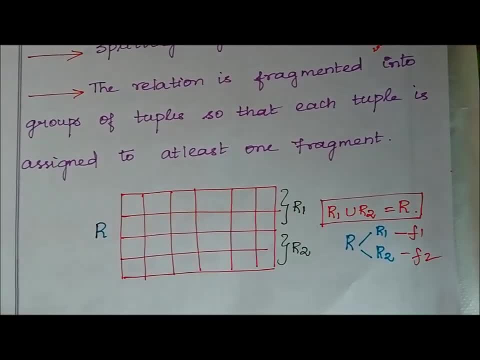 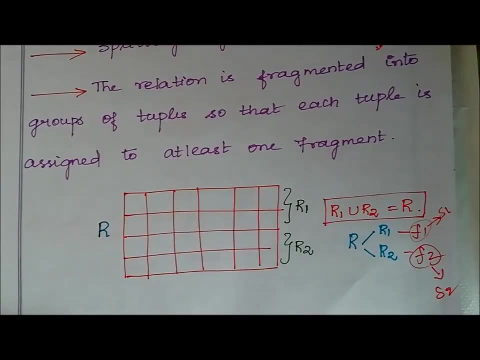 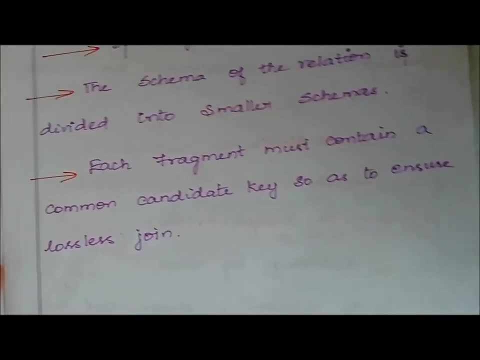 fragment- and I don't know how to win- or fragmented, okay. so either the fragment or no recital in a stupid right, consider it is yes, one fragment to in the secular store pendant. that is yes. true, this is called as horizontal frag fragmentation. okay, ma let's see what is. vertical fragmentation is splitting big. 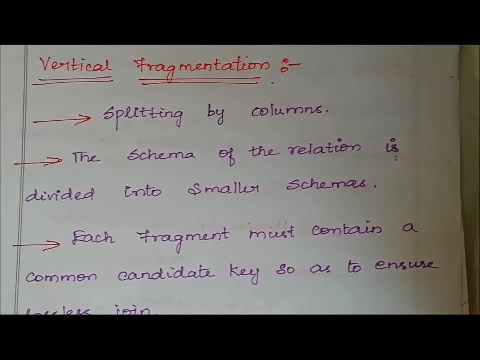 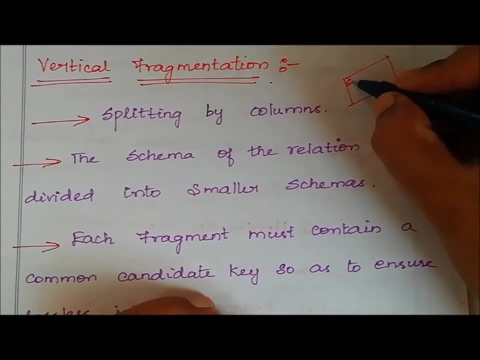 columns. the schema of the relation is divided into smaller schemas, every divided on. I prefer example number number on the path of horizontal divided by a vertical. for example, serial number: no, chakalana, I'm in the student roll number. no, chakalana. okay, student roll number. 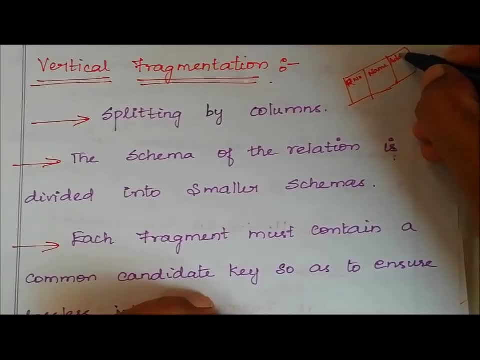 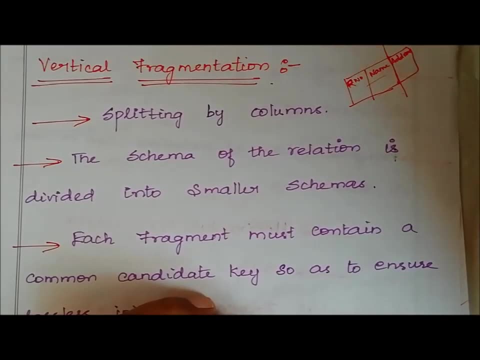 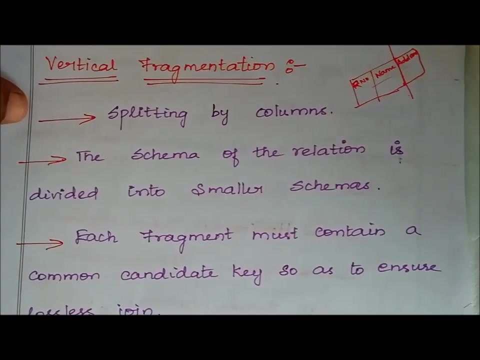 name: okay, and then address: okay. one address in which you know: okay, you slip on this smaller part on our debate, pond right, but see serial number: name over fragment on our debate, pond right. I don't understand your fragment on our debate, pond okay. so vertical fragmentation, the only opinion of Dina over a fragment. 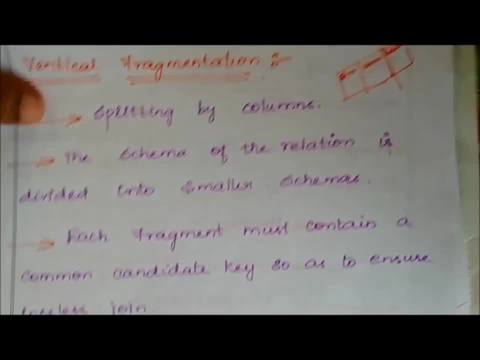 you know I'm down the fragment in surrender schemas in. so if you in a condo, Dina, when I'm in the Marty by pondering a vertical on a debate pond, right, okay. so in the my, divided by a tape or the fragment, one happens to the. 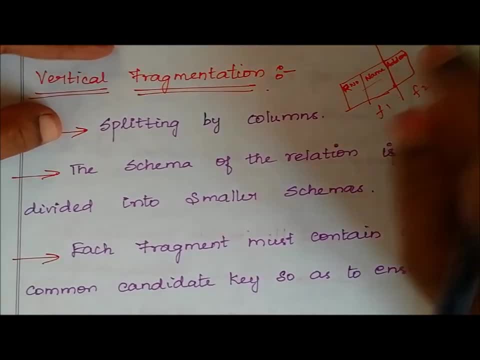 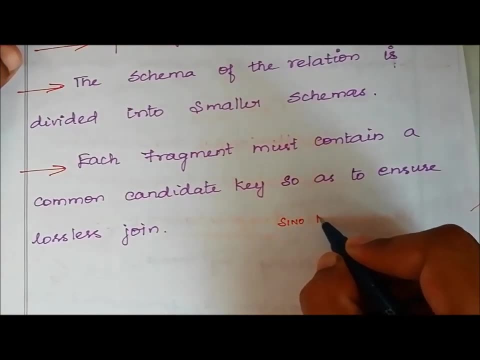 problem is fragment to weapons. 第一個 sea carbs and they're brilliant, важно gmailzeippen moment. but know, I declare me la vertical fragmentation, no willing. a Nindo nerizana first up the fragment, an insulin-c- different number and knitting divide. 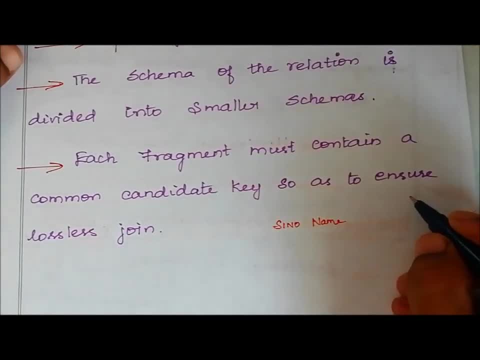 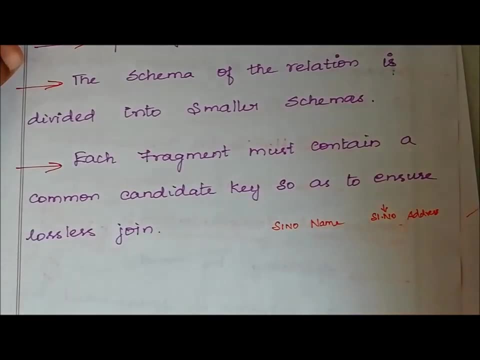 panna yama like tickler fragment pakai and then address taniaLucca now my disponibly restore or not legal number, and not that they they store okay. so Canadian��ıldÕ definition: they dry napa know how most idea story of tania venta. 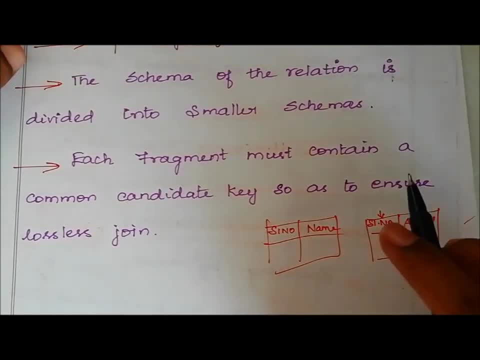 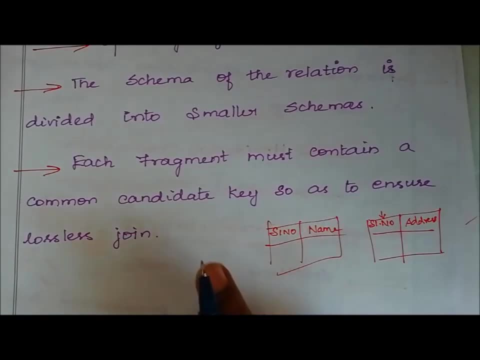 grandmother divide paname addition turned in your sinhala store. our can leave a. we will store the same key or primary key, with each attribute that we store. so why we are storing is because each fragment must contain a common key so as to ensure lossless join.